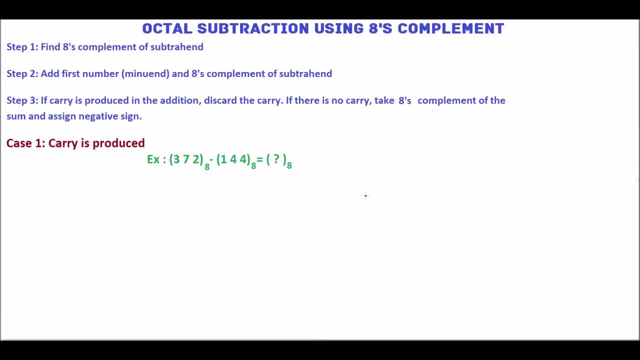 In this tutorial we will see how to subtract octal numbers using the eights complement method. We will see two different types of problems. First we will solve the example 1.. Assign the numbers as x and y for our calculation purpose In step 1, find the eights complement. 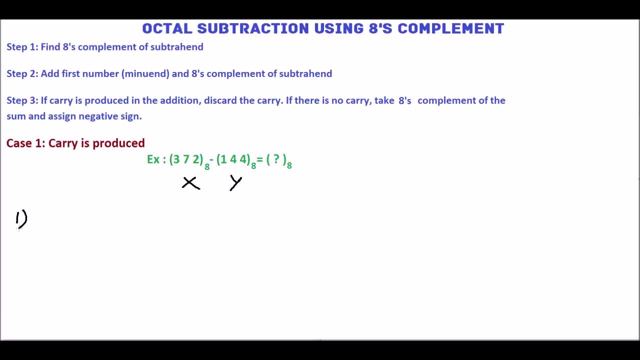 of y. To find the eights complement, first we have to find the sevenths complement For this subtract, each and every digit from number 7.. 7 minus 4 is 3.. 7 minus 4 is 3.. 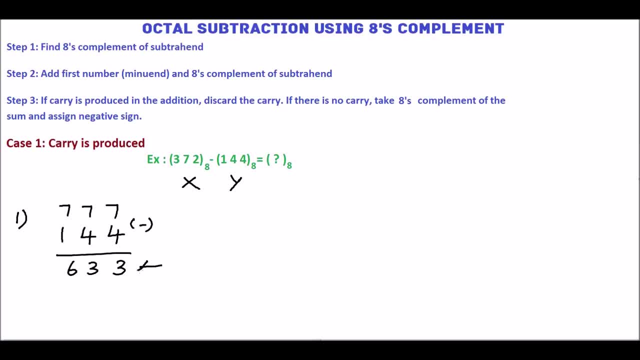 7 minus 1 is 6, which is Sevenths complement. So add 1 with this To get the eights complement. 3 plus 1 is 4, 3, 6.. 6, 3, 4 is the eighths complement of y. In step 2, add the number. 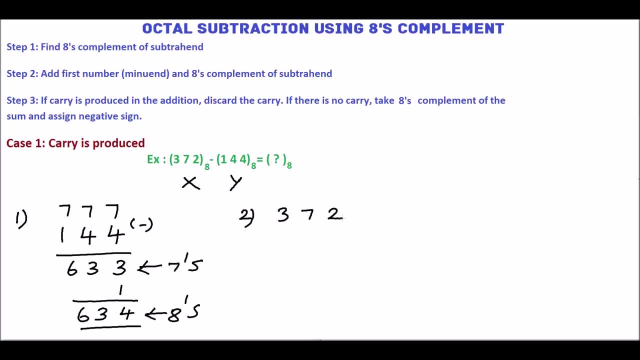 3. again To find the eights complement. first we have to find the sevenths complement of x and 8's complement of y, which is 6, 3, 4. add this: 2 plus 4 is 6, 7 plus 3 is 10. 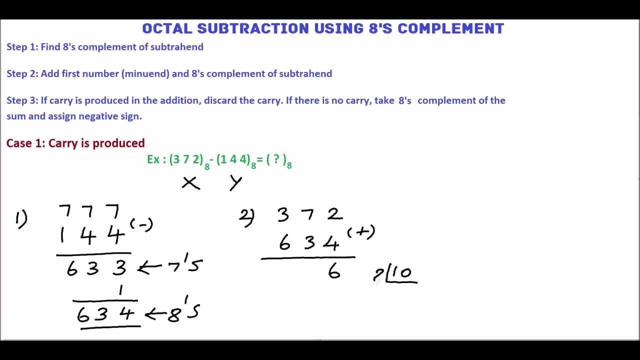 10 is not an octal number, will convert this. the quotient is 1 and the remainder is 2, so the equivalent octal number is 1, 2, 2 is the sum and 1 is the carry right. 2, 1, 1 plus 3 plus 6 is 10. 10 is not octal, equivalent octal. 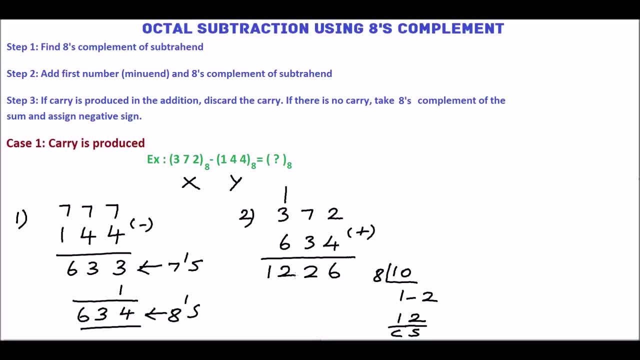 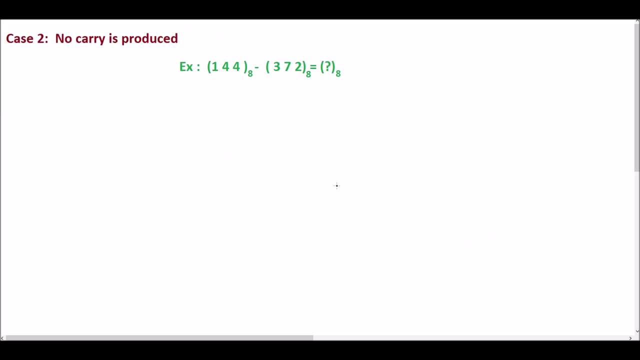 number is 1- 2. in step 2, carry is produced. this carry is called as the end-round carry. discard this carry. the final answer is 2, 2, 6. this end-round carry is the sh verification process which we shall discuss in the next A day. 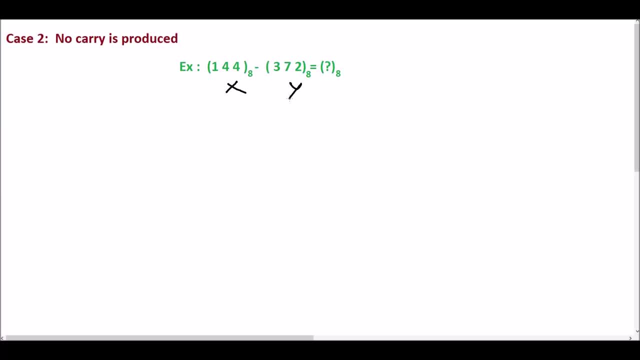 next we will move to the second example. assign the numbers as x and y. step 1: find the 8's complement of y. first find the 7's complement: 3, 7, 2. subtract the digits from number seven. 7 minus two is factory 7 minus. 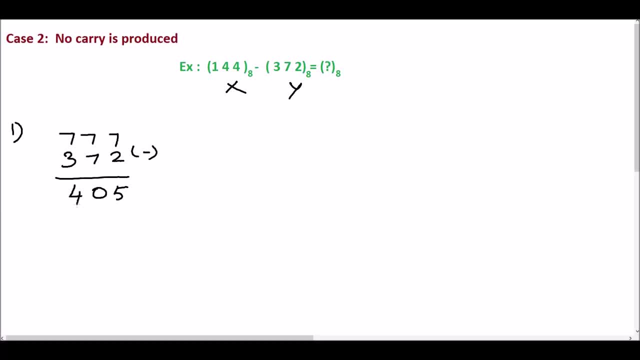 7. 7 is zero. 7 minus three is four. 7 minus three is four. seven minus 1: 0. 2, 1 minus 2 is eight. 7 minus 3 is 4. 7 minus 3 is 8 plus 2 is therefore had 8 and match theую grams are the untenorte. no doom B rabi in the math. we can use all changes for alft elect% graphic and alftятся. 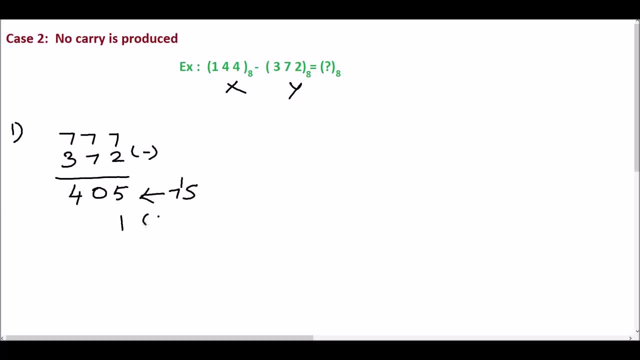 which is 7th complement. add 1 with this to get the 8th complement. 5 plus 1 is 6 0 4. 4 0, 6 is the 8th complement in step 2. add x and 8th complement of y, which is 4 0 6. 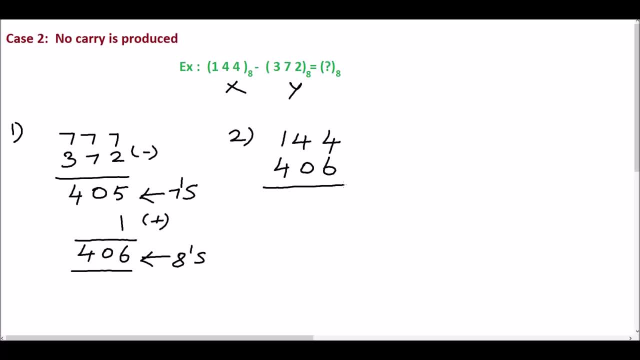 4 plus 6 is 10. 10 is not an octal number so i will convert this into octal. portion is one, the remainder is two. so 1, 2 is the equivalent octal in this. two is the sum and one is the carry. so 2, 1, 1 plus 4 plus 0 is 5. 1 plus 4 is 5. 5, 5, 2 is the sum. 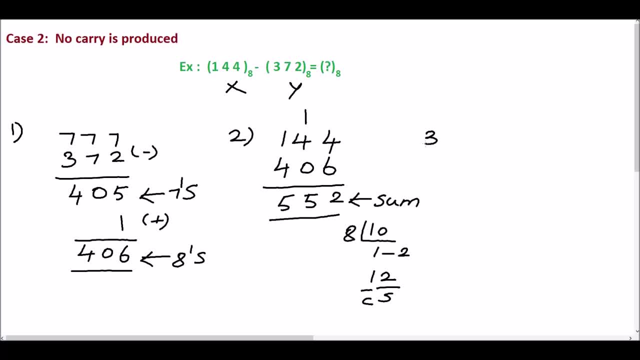 in step 2. there is no carry, so take the 8th complement for the sum first. find 7th complement. the sum is 5, 5- 2. subtract this: 7 minus 2 is 5. 7 minus 5 is 2- 7. 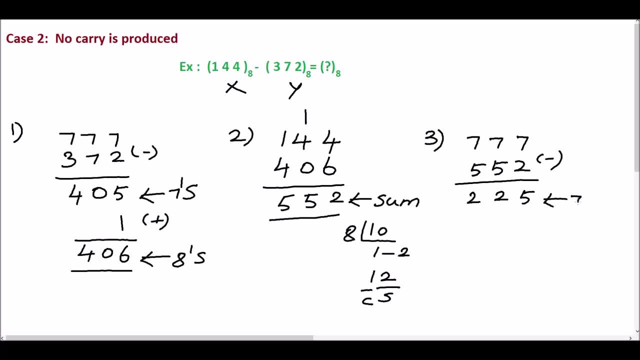 minus 5 is 2. this is 7th complement. add 1 with this. 5 plus 1 is 6, 2, 2. this is 8th complement. finally, assign the negative sign. so the answer is minus 2, 26 base 8. we will summarize this step. first, find the 8th complement for the. 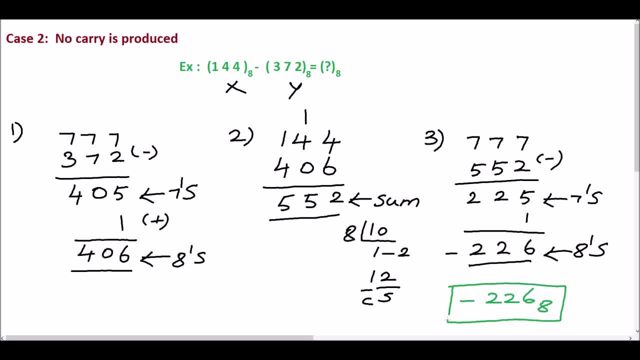 separahand, then add the first number and the 8th complement of the separahand. if carry is generated in the addition, discard the carry. otherwise take the 8th complement for the sum and assign the negative sign. thank you.